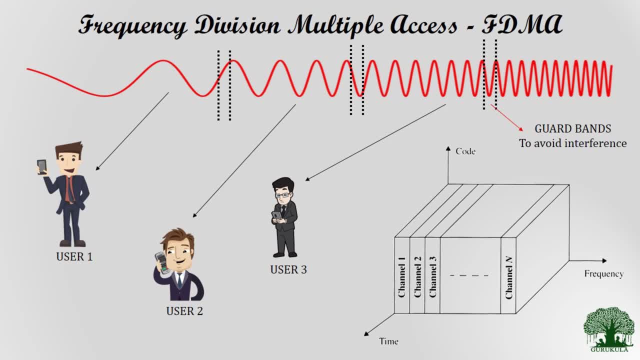 a different frequency band and then each and every frequency bands will have a gap, and that is what we call it as a god bands. and these god bands are introduced to avoid any interference between the uses. So, as you could see, or in the diagram over here, the official representation of FDMA and the uses are restricated or the uses are differentiated in terms of frequency. So this principle is what we have discussed as frequency division, multiple axis. So let's get started. 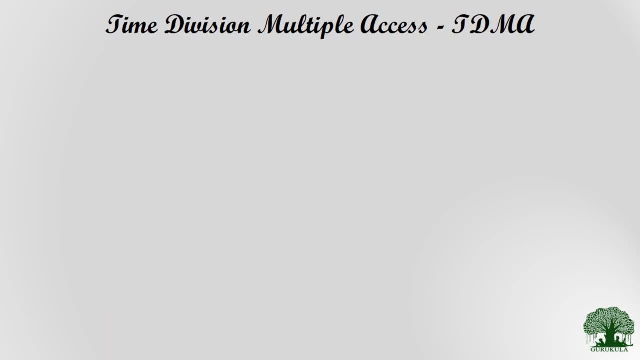 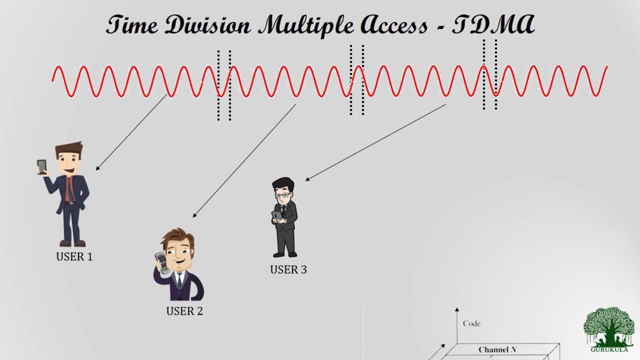 axis. so, whereas time division multiple axis is concerned, the difference is, instead of allocating different frequency bands for different uses, the entire range of spectrum is allocated for each and every user, but the differentiation is done in terms of time period, meaning each and every user will be allocated the entire range of frequencies for only a particular time period. so, as depicted, 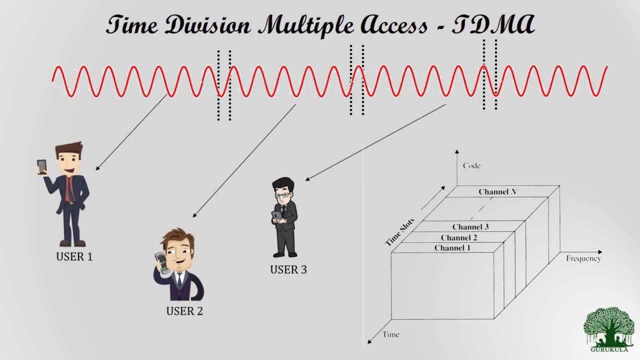 in the figure you could see that the users are differentiated with respect to time slots. so whenever the user is getting his particular time slot, he could be able to communicate the messages for the entire spectrum by utilizing the entire spectrum, so that literally any user will not have. 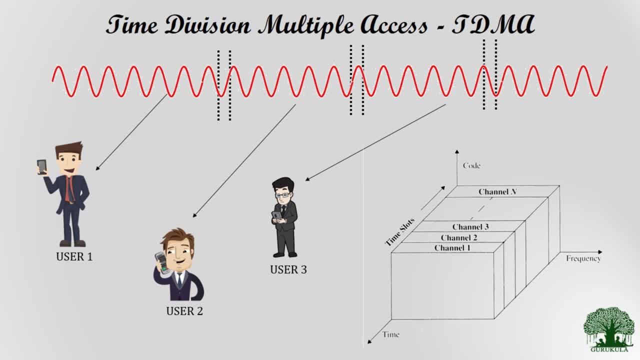 any restrictions on the band of frequencies he can use. he can use the entire frequency band, but the restriction is imposed on the time period. he can use the entire frequency band only for a particular period of time, so that he's in every time period in which every user isлучes the entire time, but the same time period in which 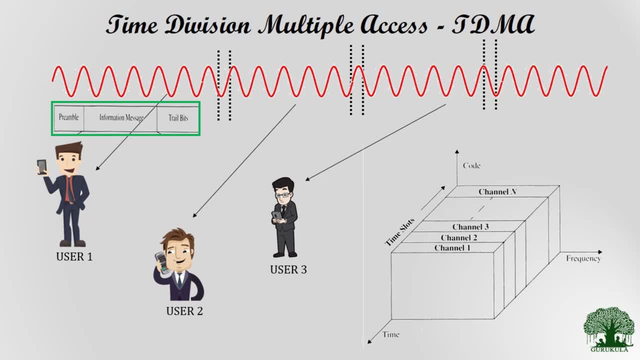 each user is getting every time slot of frequency of any of the time zones or the entire spectrum. so it is there that the user is getting the entire frequency band only so that the next user will have their own chances or their own time slots to communicate their messages, which will be added. 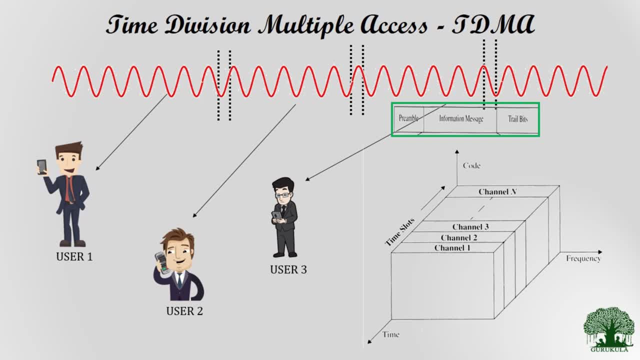 with some preamble and then trailer bits, and these tdma formats will be passed on to the next user, multiple axis. but there are certain drawbacks with the fdma and then the cdma technique. as far as fdma is concerned, the users are restricted or users are limited to particular frequency band. 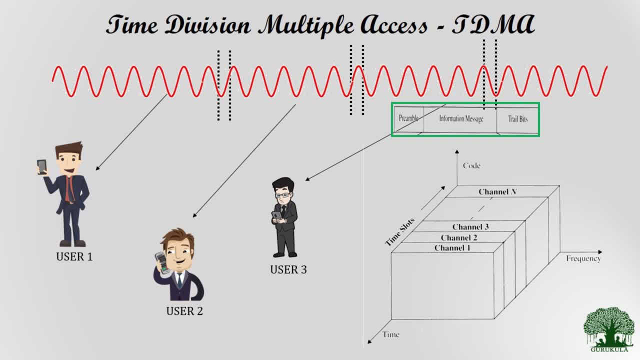 which means they could able to send on the signals that is suited within that particular frequency band. if a user wants an higher bandwidth or if he wants to communicate a very larger bandwidth of signals, he could not able to do that with respect to fdma, and whereas this 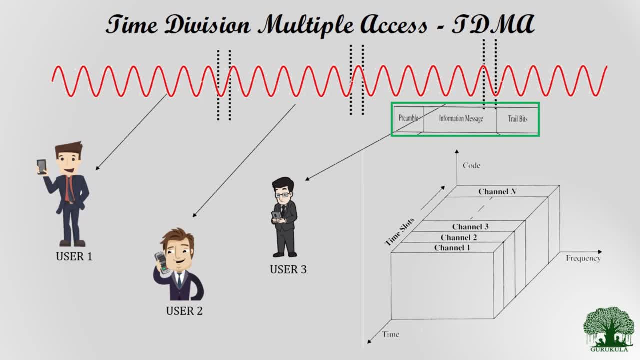 problem have been overcome in tdma technique because there is no literally restrictions on the frequency band, he can use an wideband signal, so entire frequency spectrum can be utilized by one single user at a time. but the problem comes: he can use the entire frequency spectrum only for 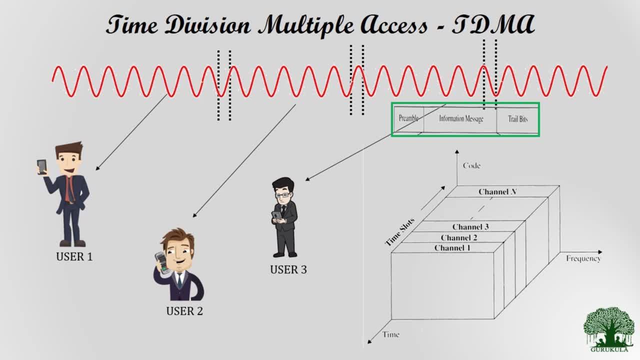 a particular period of time. so this kind of multiple axis cannot be used for continuous transmission applications. so, if at all a user has to communicate continuously and for a larger bandwidth, the tdma will also get failed. so in order to address these problems, we should come up with a particular technology where there should not be any restrictions on the frequency band and 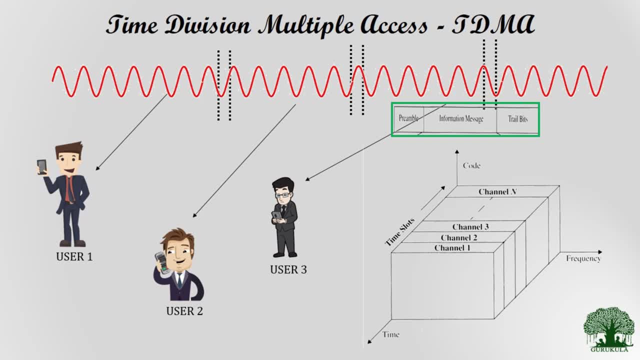 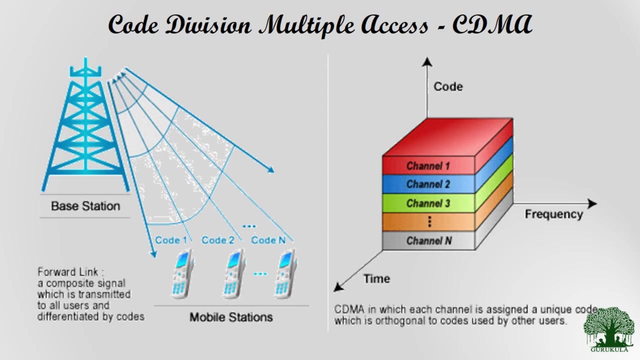 as well as the time space, but still the user has to be separated so that they can access the spectrum simultaneously. so such kind of special multiple-axis technique is what we call it as code division multiple-axis. so here in code division multiple-axis, as you could see, each and every mobile stations are: 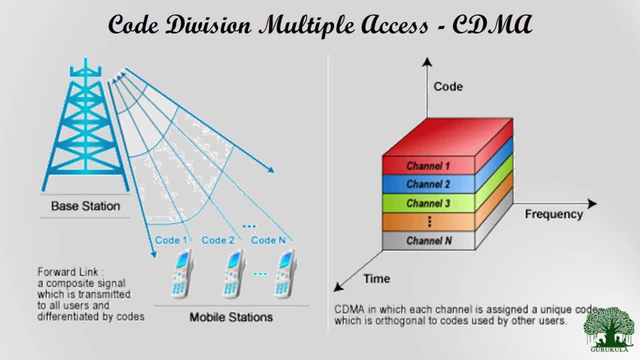 allocated a different code. so this code actually differentiates the mobile uses. so each and every user on a network connected to a particular base station will be separated by a special code. so since it is separated by a code, we call this as code division multiple-axis. so when you look at the official diagram over on the right hand side, 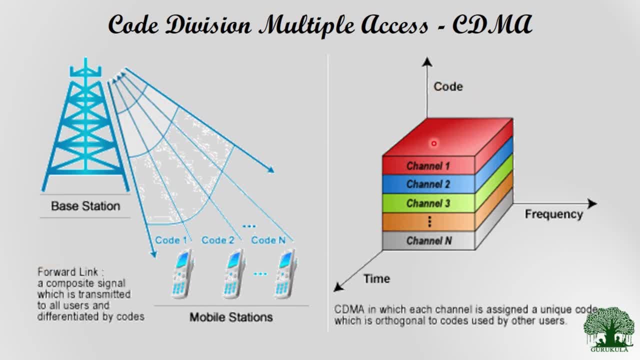 you can see that the various uses are differentiated with respect to code, so that the users are not restricted with respect to frequency, meaning that he can use the entire frequency spectrum that is available, and also he is not restricted on the time period, so that he can use the entire frequency. 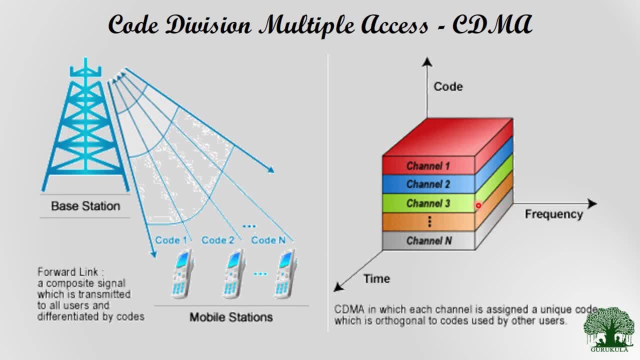 for the entire time period and then so each and every user will be allocated or differentiated with the code, so simultaneous transmission by all the users is possible. so that is the key advantage of CDMA technique when compared to FDMA and then TDMA technique. so this basic principle is: 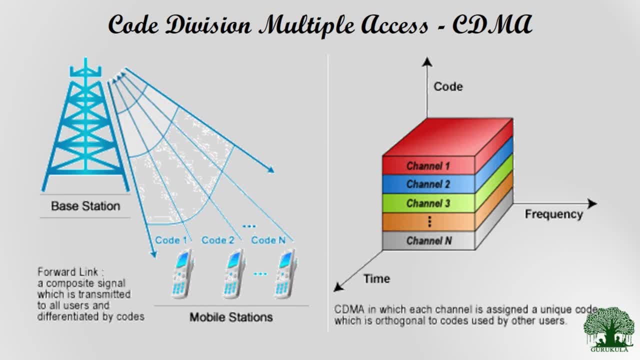 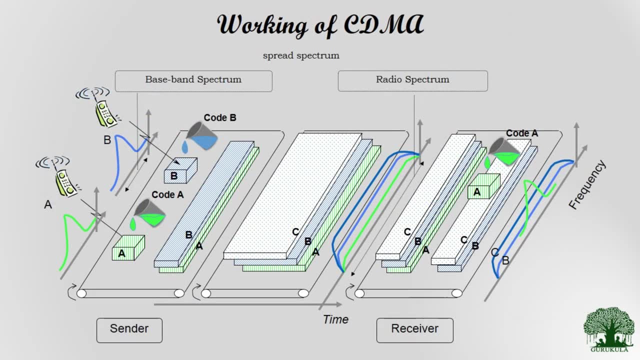 what we call it as code division: multiple-axis, where each and every user is separated with a code instead of time and frequency. so this is a basic working principle of an CDMA, where this particular diagram can help us to understand what actually happens. happens in cdma transmission. so let us consider that there are. this is the transmitter side there. 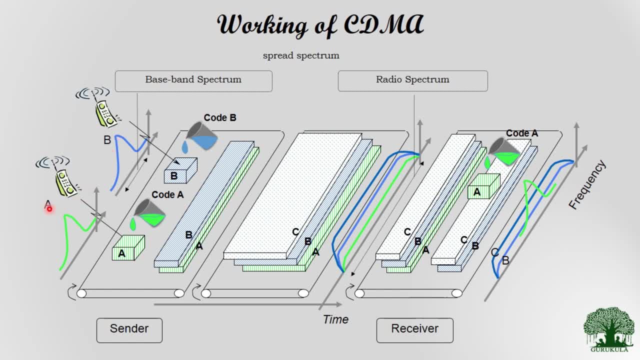 are two users. let us take a and b. so a will be generating the messages, which will be a narrow band signals, which is represented green in color, and then b will also generate their own messages, which will also be an another narrow band signal with that is represented in blue in color. so what? 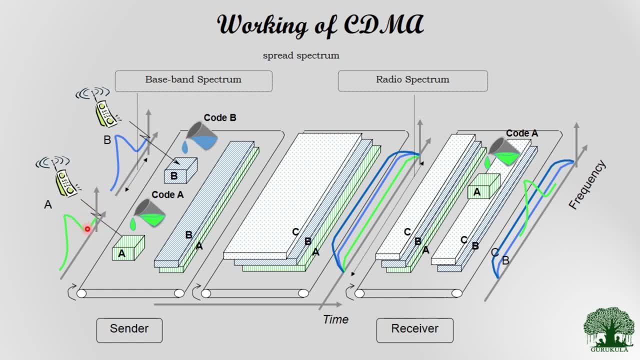 will happen is, before transmission, all these signals will be multiplied with an unique code. we call that as pn sequence code. so and these code, when this narrow band signal is getting multiplied with this pn sequence code, and these narrow band signals will be converted to a wide band signal, as depicted in the figure over here. and similarly, the same process will be applied. 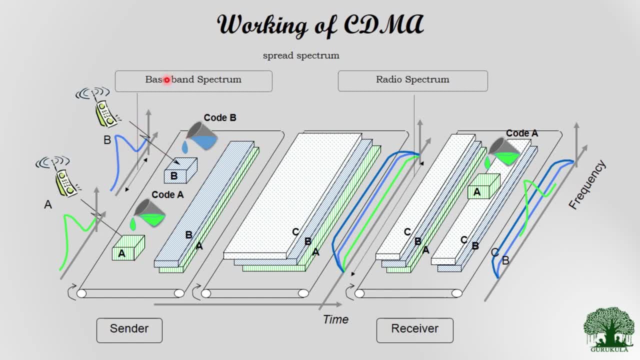 for n, a number of users. they are in the system, as you could notice, that the code a is different from code b, so each and every users will be differentiated with the code. that is the basic principle behind cdmas. so when the codes are getting multiplied, with the narrow band signals generated by the user, the 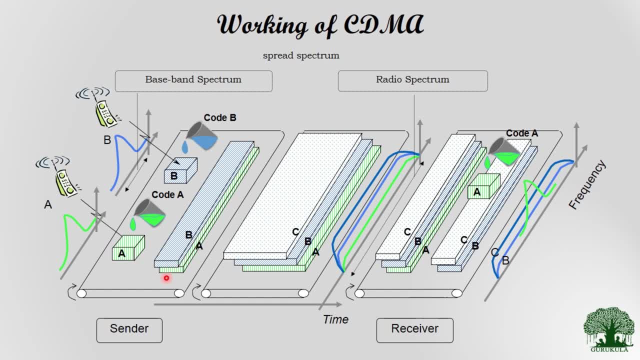 narrow band signals will be converted to wide band signals and all these wide band signals will be transferred over a radio spectrum. that is my channel. so this is how each and every user signal will be sent: over a channel and that can be replicated over here. as you could see that each 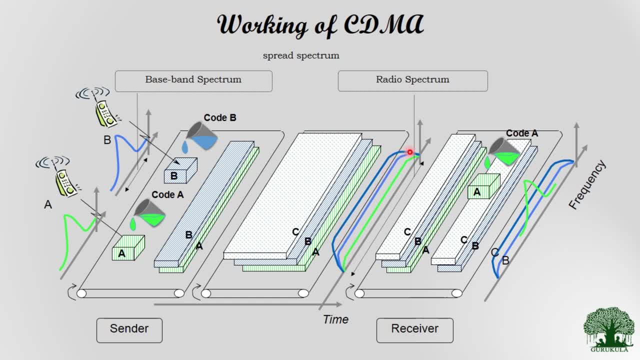 and every user will use an wide band signals over here and at the receiver side. if at all. i wanted to decrypt only the signals of user a, then i should use the same code, whatever i've used at the transmitter side, so you can observe that the at the transmitter side, the green color code, that is, the code a, have been used. 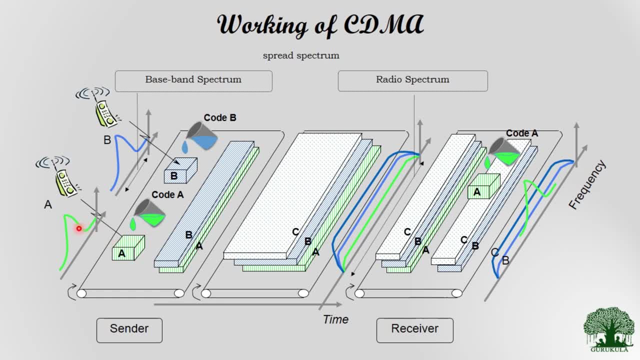 to convert or to multiply the signals generated by the a, the same code has to be used at the receiver side as well. doing so will again convert back the wide band signals to a narrow band signals, and all other remaining wide band signal remains as such, so that only this particular 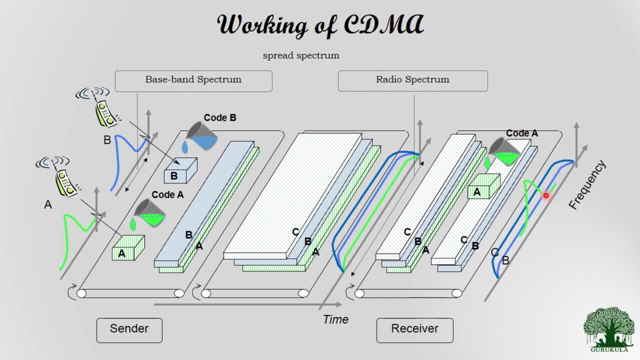 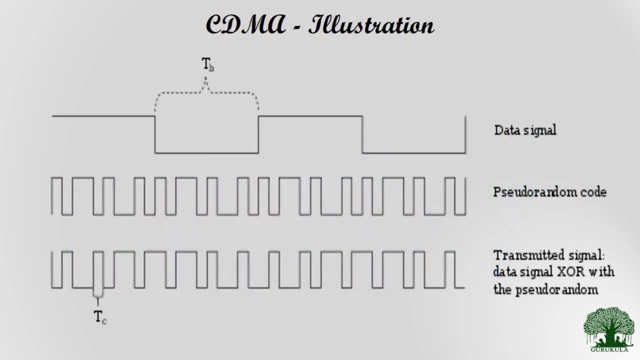 frequency can be extracted back and it can be processed to further data replication processes. so this is the working principle of an code division multiple access. so this diagram actually shows you an basic illustration of code division multiple access. so the first waveform, this is nothing but the data signal, whatever been generated by a particular 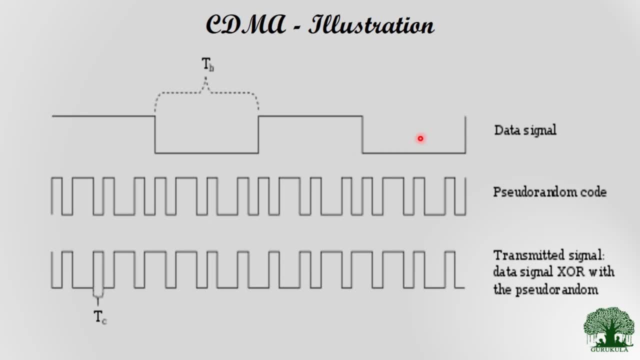 user and, as you could see, that this is an narrowband signal, and then all these narrowband signals will be multiplied with an pseudo random code. that is my pn sequence code and the. when i multiply these two signals, i will end up with a signal something like this, and it is clearly noted. 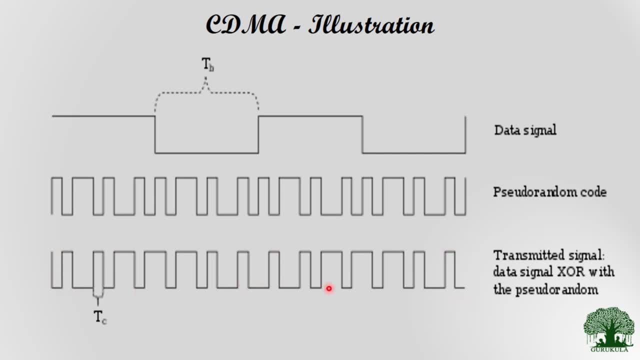 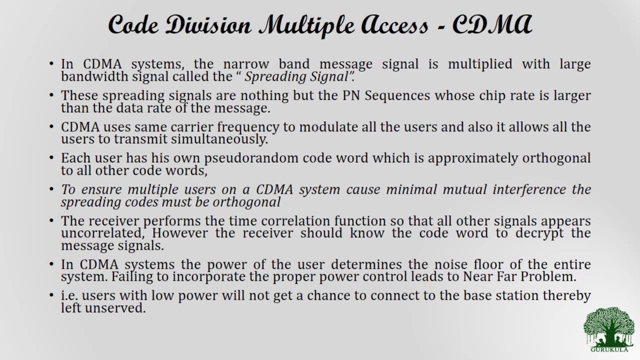 that these signals are the wide band signals, and this signals is what actually we call it as encoded signals, and these encoded signals are only transmitted over the radio channel. so that is an basic illustration of code division, multiple access. to sum up, the code division, multiple access systems, the narrowband messages, whatever been. 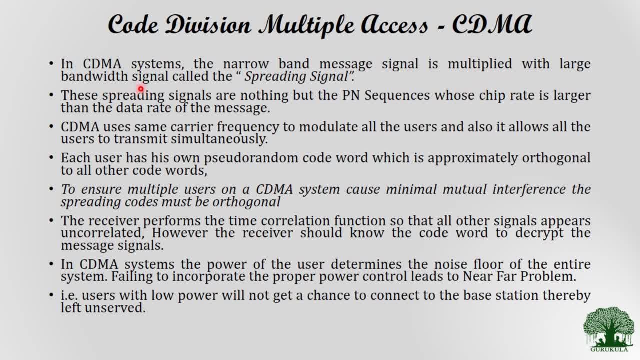 generated by the users are multiplied with a large band signal and we call that as spreading signals. so actually, the signals are getting spreaded and the narrowband signals are converted to wide band signals. so the way, the key principle, is what we call it as signal spreading and this spreading 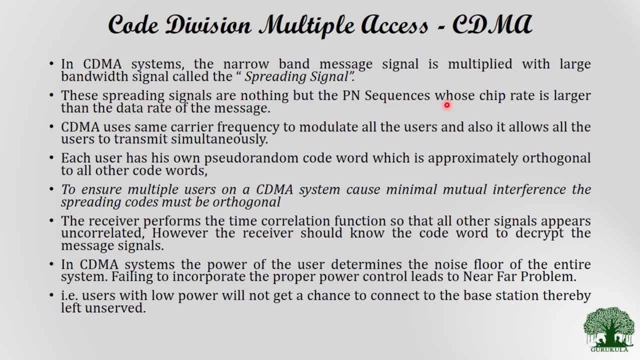 signals are nothing but the pn sequences whose chip rate is larger than the data rate of the messages. and then the code division. multiple access uses the same carrier frequency to modulate all the uses and also it allows all the users to transmit simultaneously. and we also know that from the 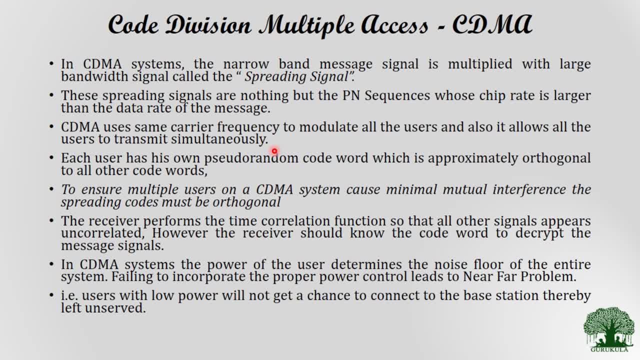 formal representation of cdma diagram. we have seen that there is no restriction for the uses on frequency part and as well as the time part. it, since each and every uses are differentiated with the code, all the users are allowed to transmit their messages simultaneously over the, over the common radio spectrum and then 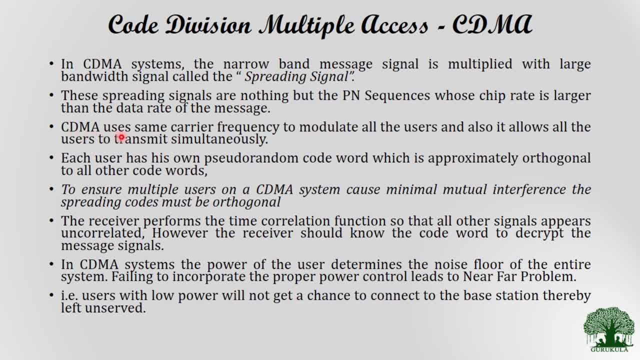 it is important to note that the cdma uses the same carrier frequency to modulate all the uses. so this point will be stressed again when we are discussing the topic of dma. so there the difference will be coming. when, what? what will be the difference for using the same carrier frequency? 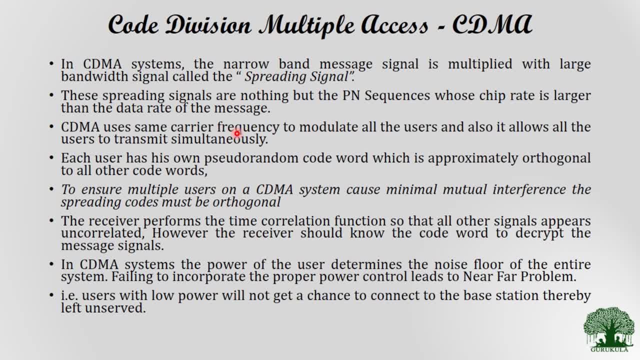 and different carrier frequency. so as of now, it is just requested to note down that the cdma uses the same carrier frequency to go against the normal radio spectrum. you can see that we are resort to that string that we are going to use for conducting the following 3D Photo. 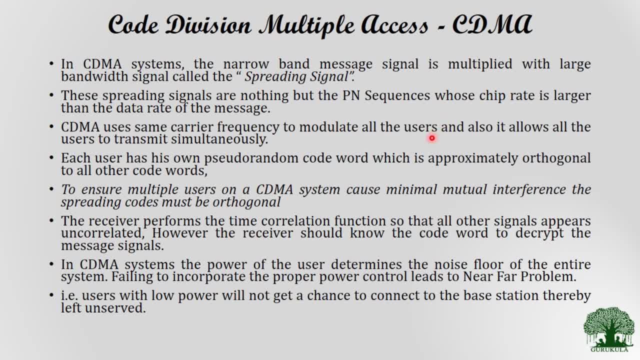 so information is must be stored within the carrier frequency. so the Gaussian diffusion free filter we are producing is about railroad frequency, and this goes a way beyond what non-physical applications actually Terrace URI represents. so if you are looking for a random code word in our country, simply go to the keyword library or in the youtube. coach셨�ocom. 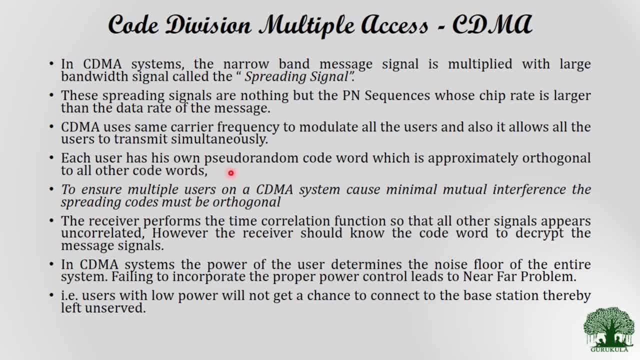 or orthogonal to each other. so the meaning for orthogonal: it can be defined in multiple ways. in general everyone will say the 90 degree phase shift is what we call it as orthogonal. but in general orthogonality can be stated as any minimum deviation that is required. 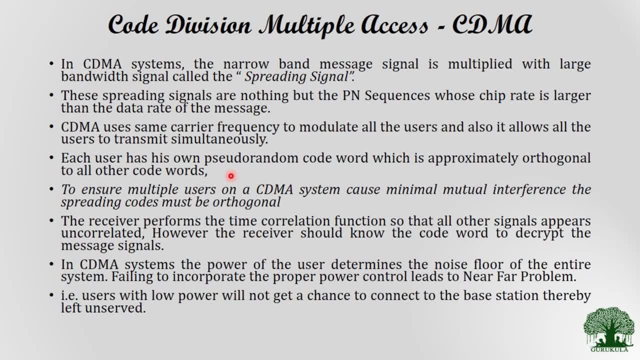 in order to differentiate two different signals without any interference is what we call it as orthogonality, or from the physics. take, for an example: there are two codes and when you take a dot product of these two codes, that should result you in zero. so if this condition is getting, 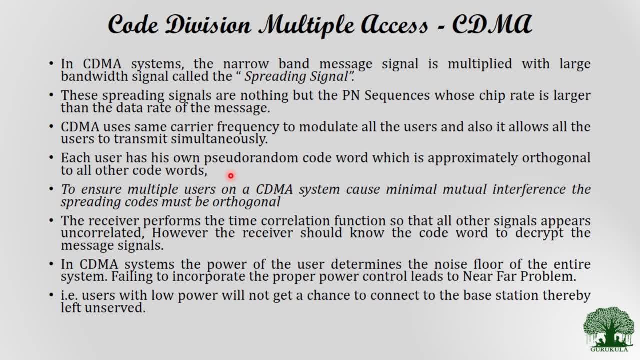 satisfied. we can call that, as the codes are orthogonality, so this principle is what we call it as: orthogonal and, however, orthogonality principle will be revisited again when we are discussing OFDMA, but as of now, we should understand that orthogonality is a principle which should be. 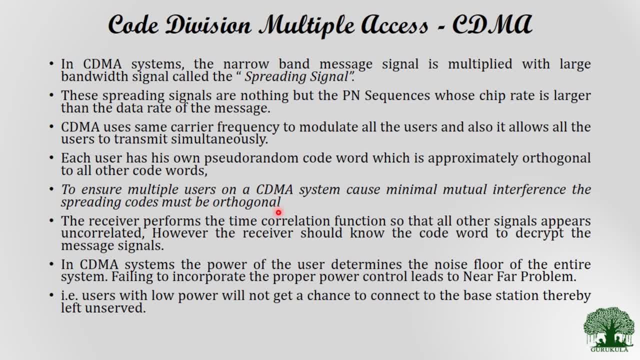 maintained. maintained between the codes, that meaning that user A and user B will have two different codes and these two codes should be orthogonal to each other. So bringing orthogonality among the codes will make the signals of user A and user B to be very much uncorrelated. So bringing in the 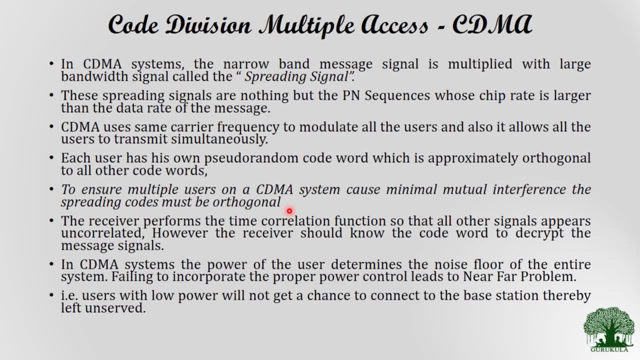 uncorrelation among the signals is an important parameter to reduce the interference in the transmission system. If at all the signal seems to be very much correlated, then that gives you the meaning that the signals are very similar to each other. then that will lead to intersymbol. 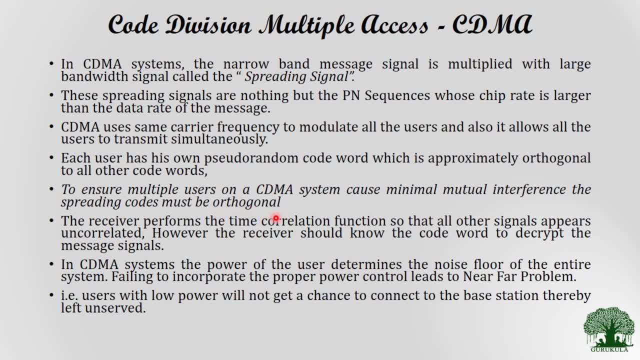 interference. So actually bringing in orthogonality among the codes is very important parameter and it is mandatory to have the orthogonal codes in the system. So code A and code B should be orthogonal to each other and, however, no matter how many number of codes we are using, we should 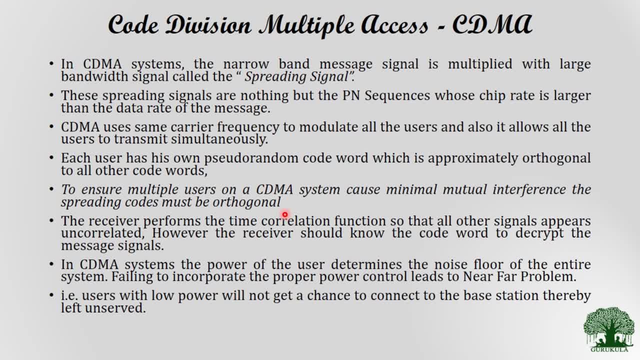 have an orthogonality among the codes That we use for transmission and receiving purposes, So the receiver performs the time correlation function so that all other signals appears uncorrelated. however, the receiver should know the code word to decrypt the message signals, So that is actually known to us while discussing the working. 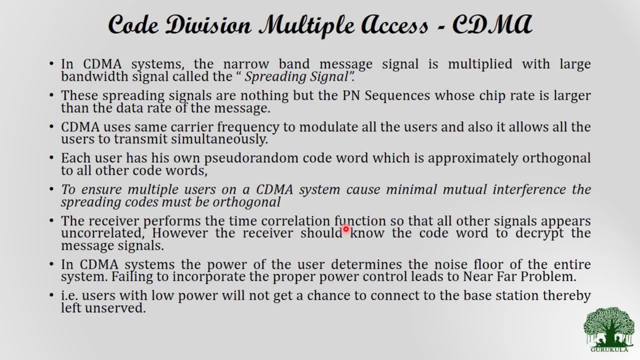 principle of code division: multiple access when we have to, when we can actually decrypt the messages effectively only if the receiver knows the code word That is used for encrypting the messages at the transmitter side. In CDMA systems, the power of the user determines the noise floor of the entire system, So failing to incorporate the proper power control leads to near 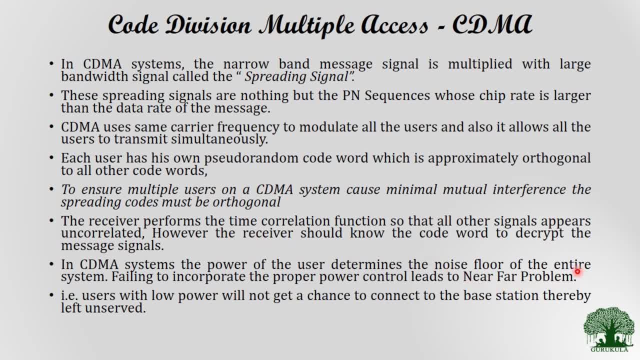 far problem. So this is a very serious issue which has to be addressed in the CDMA technique, whereas we could say that this is the drawback which the code division multiple access faces. However, the code division multiple access overcomes the drawbacks that we faced in previous techniques, such as FDMA. 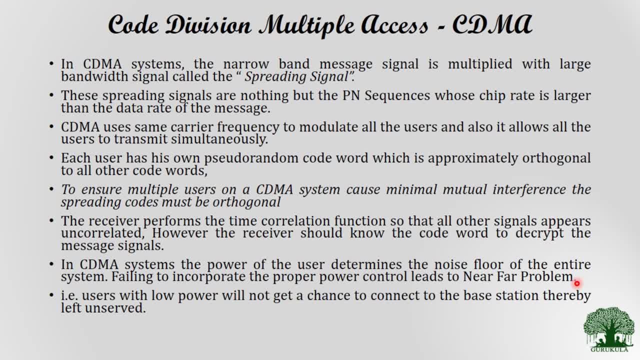 and TDMA. There are certain drawbacks with the code division, multiple access as well. One among those drawbacks are this near far problem, which can be controlled by using a proper power control mechanism. So that is say, for an example, if the user with low power will not get a chance to connect to the base station, thereby these users 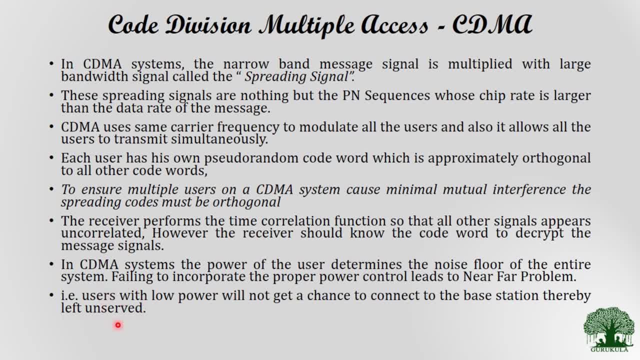 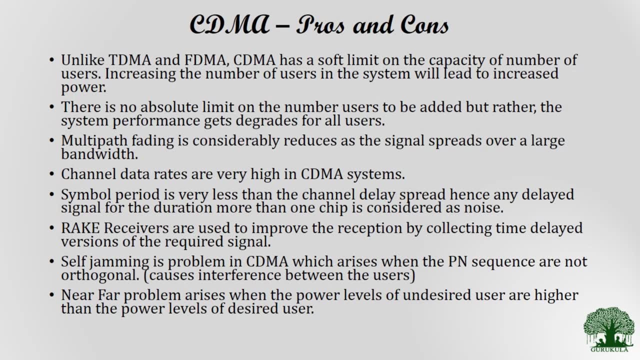 will be left unserved, And this particular scenario is what we mean to as near far problem. So we will try to go in detail about this near far problem in the next slide, where it will be, where it will be depicted with the figure. Actually, there are certain pros and cons when compare for the CDMA technique, unlike CDMA and FDMA, sorry. 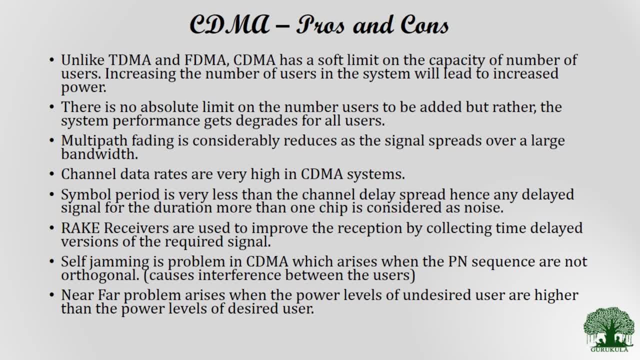 unlike TDMA and FDMA, CDMA has a soft limit on the capacity of the number of uses. Actually, you do not have any hard limit on the number of uses. So if you have a hard limit on the capacity of the number of uses, actually you do not have any hard limit on the 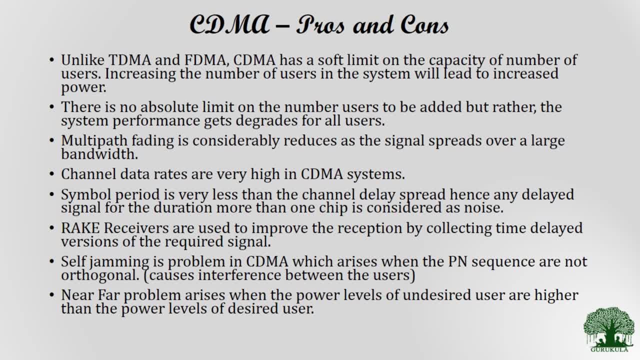 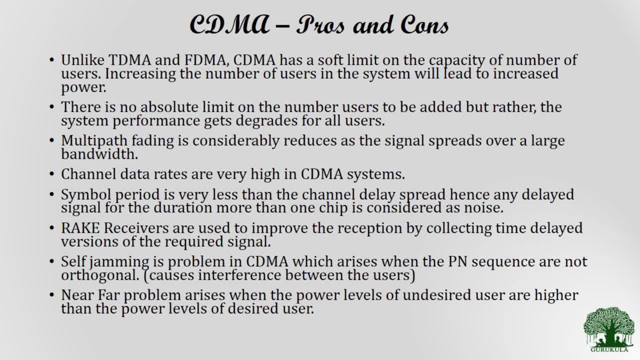 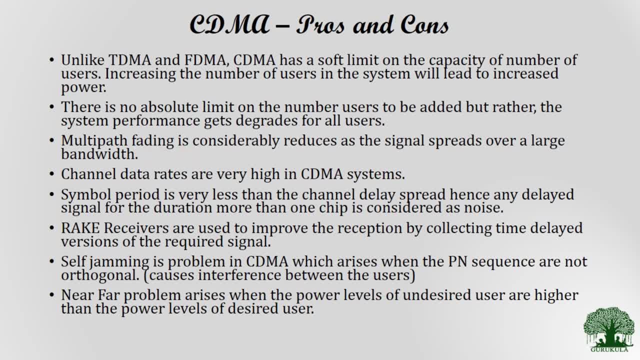 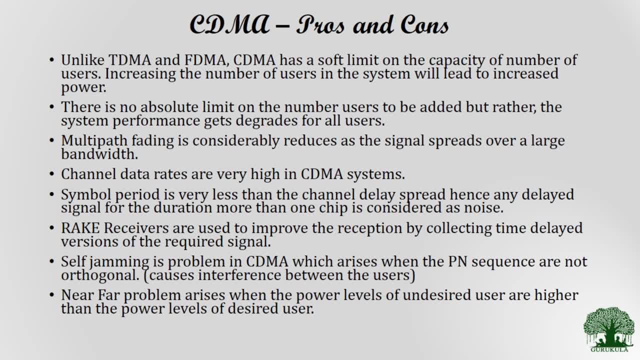 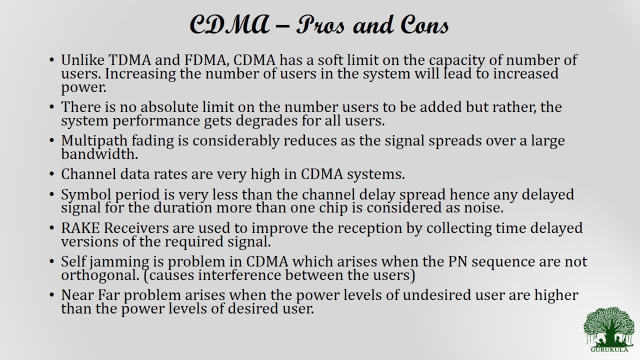 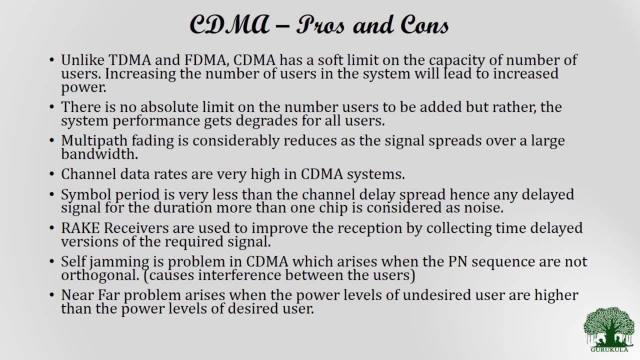 that are delayed in time. so rake receivers are effective in receiving the signals which are, which have different time periods. self jamming is a problem in CDMA which arises when the PN sequence are not orthogonal. so, as it is already discussed, the orthogonality among the signals has to be maintained. 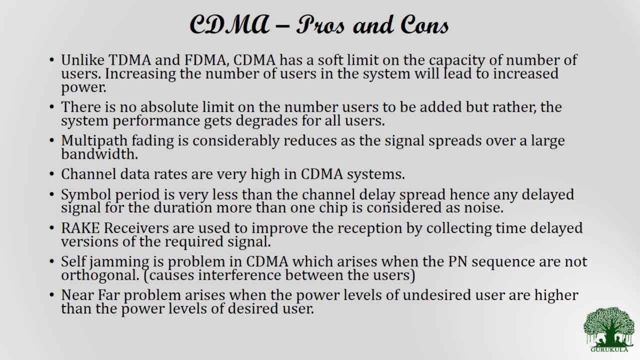 if it is not maintained properly, then that will lead to interference between the uses. and the final last and drawback is the near for problem which will arise in the power levels of undesired user or higher. so now it's time to discuss what near for problem is actually and when does the near for 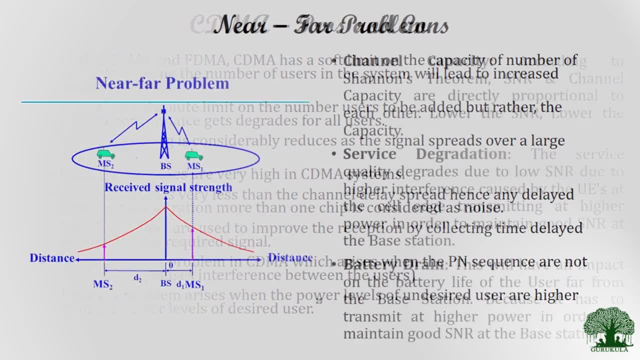 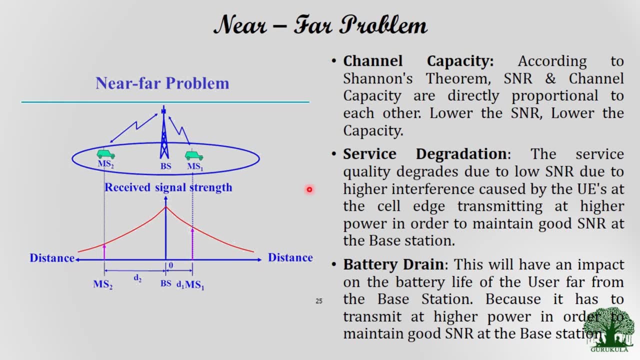 problem actually arises. we will see in the next slide. so let us consider that this is an near for problem illustration. so when you observe this particular figure, we could see that this is the base station which is serving and geographical area that is marked like an circle over here and you can. 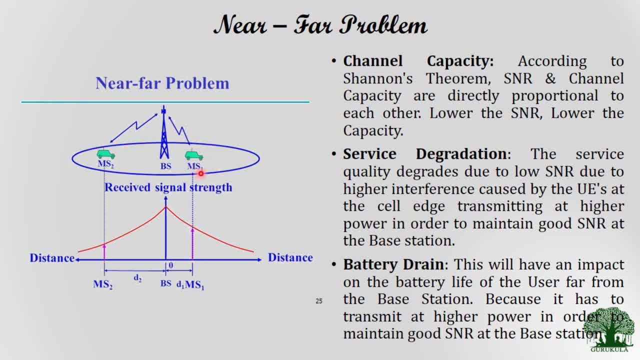 observe that we have. we have two mobile stations, ms1 and then ms2, and it is observed that ms1 is very closer to the base station and ms2 is far to the base station. so let us consider that now my ms2 is the desired user, which I wanted. 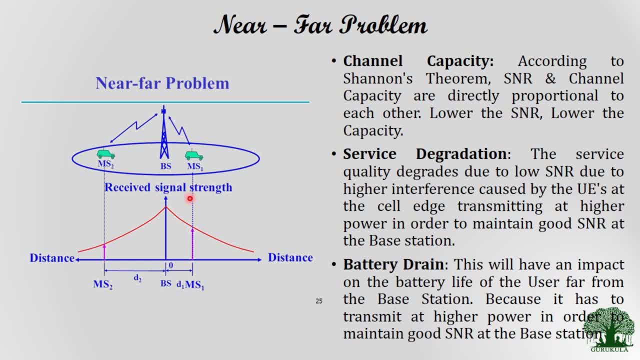 to serve now. so when I look into the received signal strength graph, so where I will take distance on the x-axis and the received signal strength on the y-axis, so this actually the signal strength that is depicted for ms1, that is, your mobile station 1, and we know that from the basics of the wireless propagation. 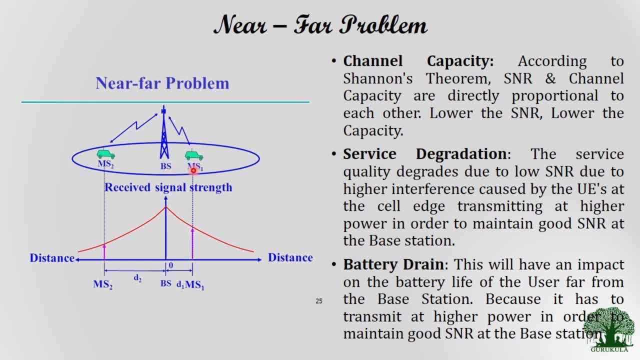 models. when the distance between the base station and then the mobile station is increased, then there will be an degradation in the received signal strain. so that is what is depicted over here and, as of our example is concerned, ms1 is very closer to the base station, so that it will have higher power when 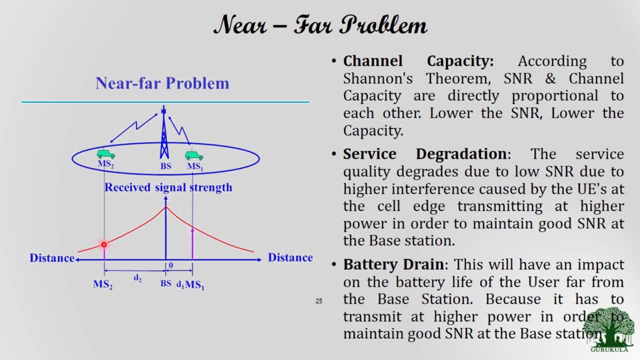 come as as and the mobile station 2. So mobile station is very far from the base station, so that at this particular distance the received signal strength will be very much lesser as compared to your mobile station 1.. So this problem actually leads since the MS2 is not having proper power levels. 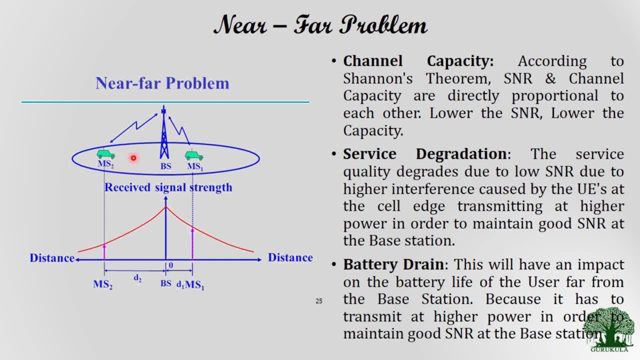 or the signal strength to reach with the base station, this MS2 can be left unserved. So this problem is what we call it as near-far problem. So in order to overcome this near-far problem, the only way that we use is this: mobile station 2 should transmit with an higher power in order. 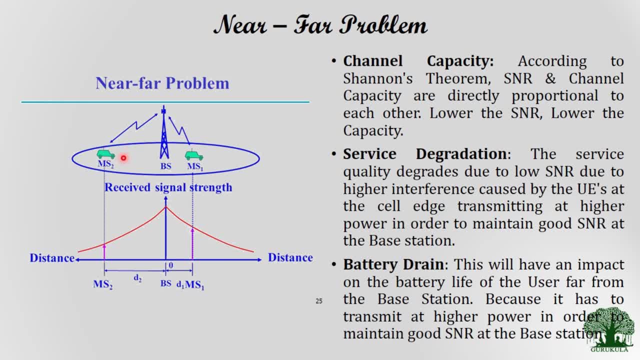 to compensate this particular distance. So if we use higher power then that will actually degrade the battery performance and more power consumption. So this is an cyclic process and these are all the effects of near-far problem. So we could see that there are three drawbacks. 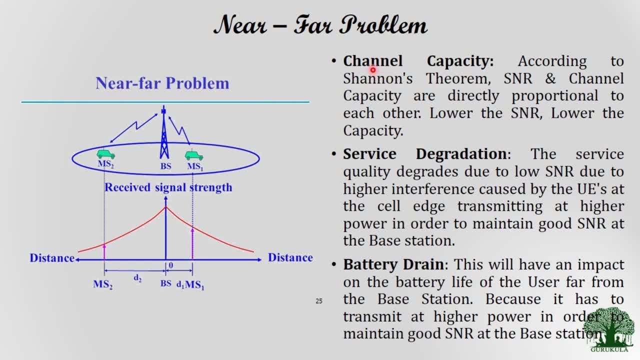 when we are using a mobile station 2.. So the first one is that the mobile station 2 is not having proper power, which could arise because of this near-far problem. The first one is channel capacity. So, as per the Shannon's theorem, signal to noise ratio and channel capacity are directly. 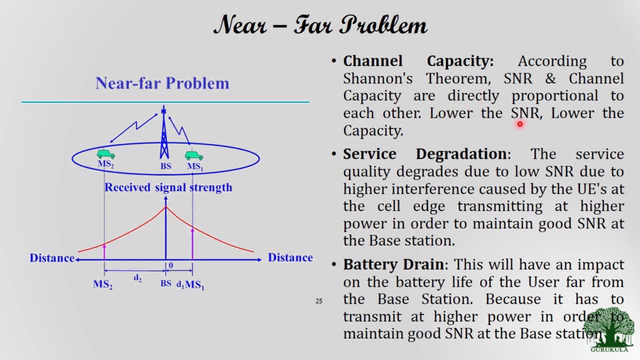 proportional to each other. So lower the signal to noise ratio, lower the capacity is So in order. so we have to try to keep the signal to noise ratio at an optimal level. And signal service degradation. So service quality will degrade due to the low signal to noise ratio. due to high interference caused by the signal to noise ratio. So this is a problem which could arise because of the high frequency of the signal to noise ratio and the high frequency of the signal to noise ratio. So this is actually a problem where the entire signal to noise ratio is caused by user equipment. 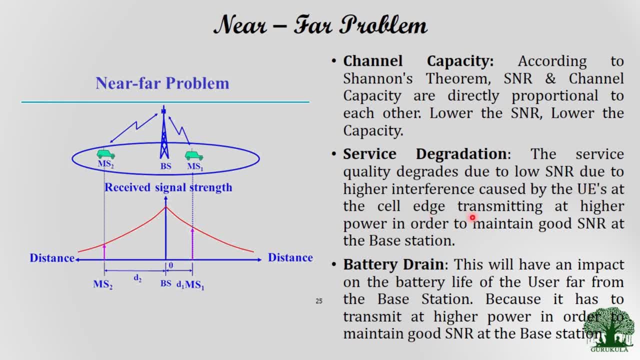 So UE stands for user equipments at the cell edge, transmitting at higher power in order to maintain the good SNR. So this is what actually we have discussed. So in order to maintain a good SNR signal to noise ratio, this MS2 is forced to use high power levels to transmit their signals between 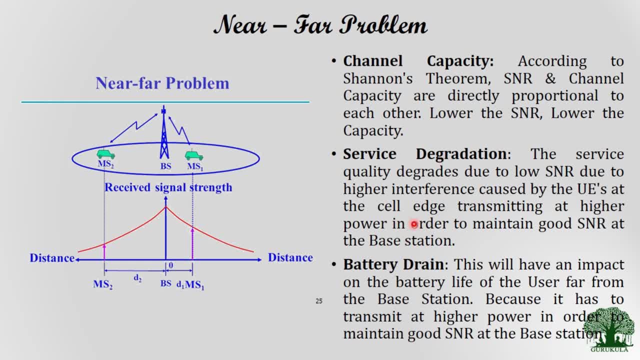 the mobile station and then the base station. So this is what actually leads to service degradation. So, since this is using high power, then there will definitely be battery drain. drain, sorry. so. each and mobile devices are powered with an battery pack that we hold in our hands, so 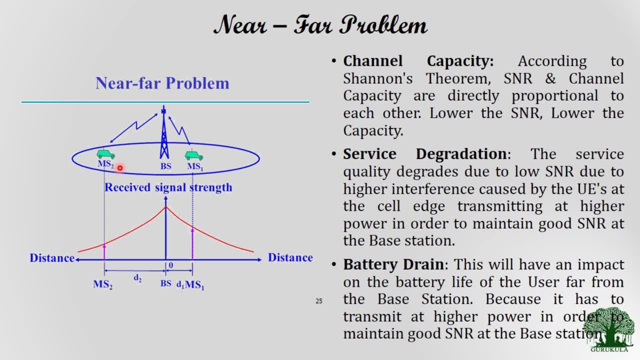 that is powered by an battery pack. your more battery life will be affected when the user is far away from the base stations. so it is quite natural that it is already known that when the signal level, so the received signal strength, are very less, our battery will drain as fast as. 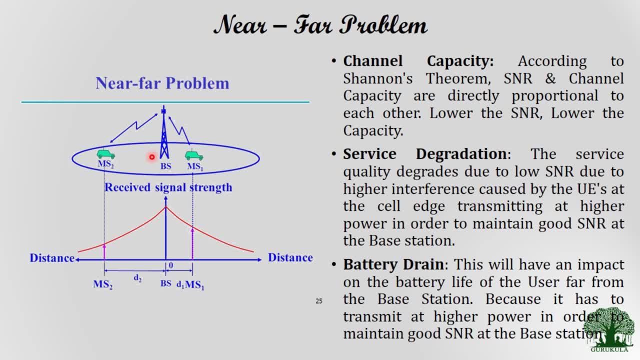 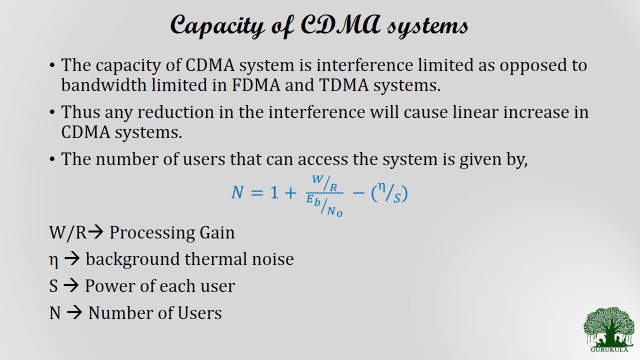 possible because it is transmitting the signals with high power, so that requires higher energy, that will consume more power from the battery. so these are all the major problems that is arised because of the near for problem. so this drawbacks has to be addressed effectively while designing the code division multiple axis system. so then to talk about the capacity of 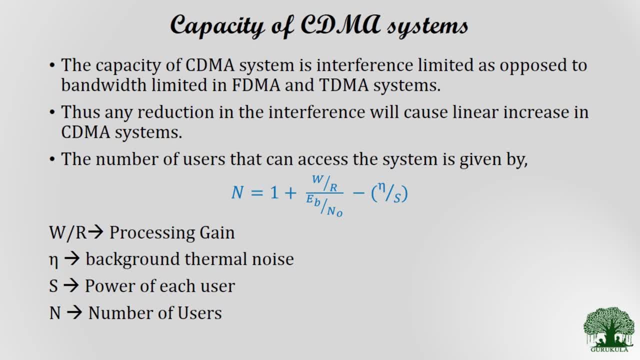 code vision multiple axis. we said that there is no hard limit on the number of uses that can be incorporated into a CDMA system. however, we cannot include an infinite number of of users in an restricted code division multiple access system, since it degrades the performance of 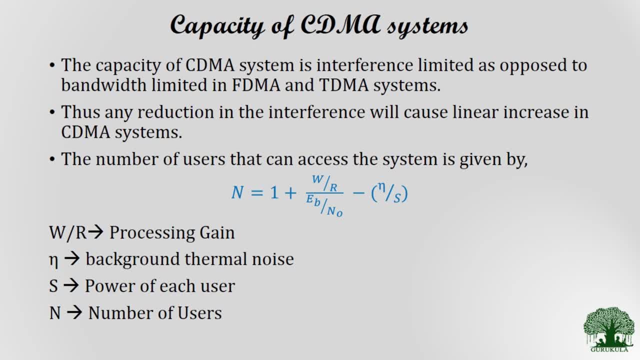 the entire system, the actually the performance will be degraded for each and every user present inside the system. so it is always better to have a limit, an appreciatable limit or acceptable limit, where the number of users that can access the system at the same time is given by the equation. 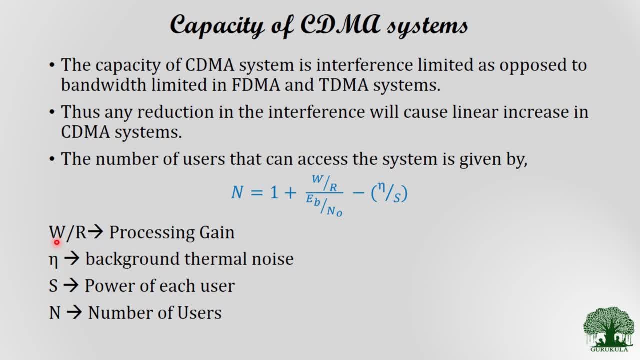 which is shown over here, and where w by r represents the processing gain and where eta represents the thermal noise that is present in the background environments and s is nothing but the power that is generated by each and every user and n represents the total number of uses. 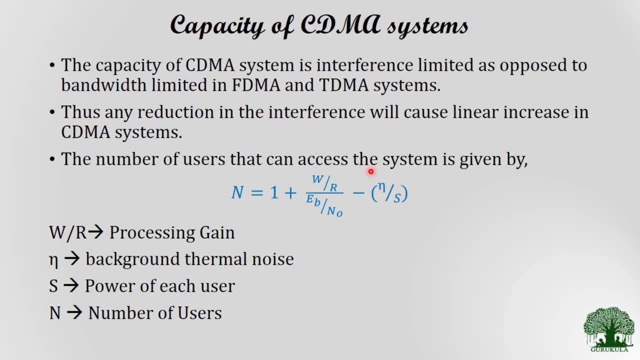 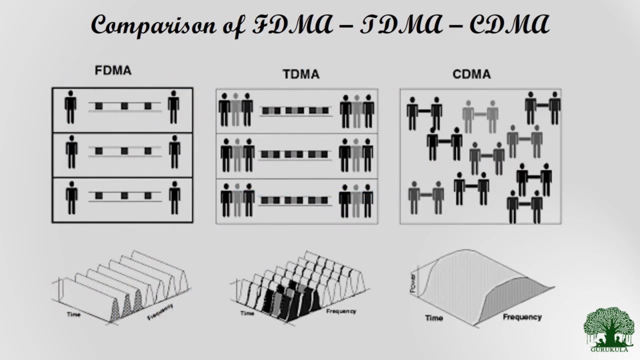 so we have to satisfy this particular equation so as to decide what will be the total number of users that can be effectively allowed to access the code division multiple access system. so this is all about the code division multiple access system. so now, when we try to compare, 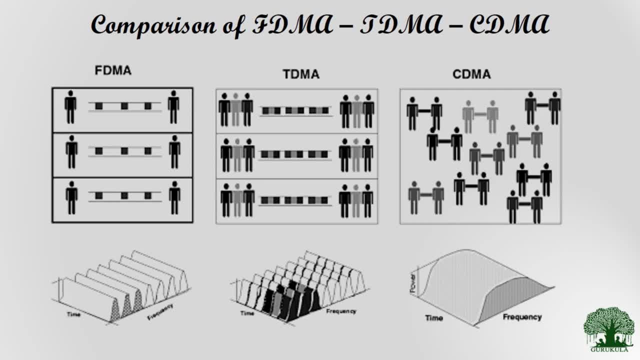 uh, the techniques, whatever we have seen, that is uh: frequency division- multiple axis, time division multiple axis and code division- multiple axis. in fdma system, each and every user will be allocated a different frequency band and then, so users are not resticated on time, they can use the smaller. 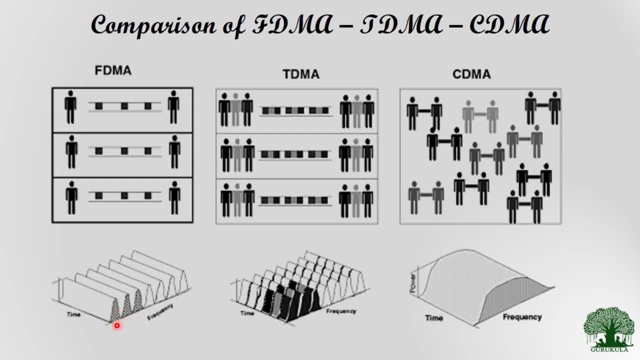 frequency bands whatever being allocated to them for the continuous period of time. the drawback with fdma is a user could not able to send or receive the signals in a larger bandwidth if he has to be transmitted with a larger bandwidth. that is not possible with fdma systems, but continuous. 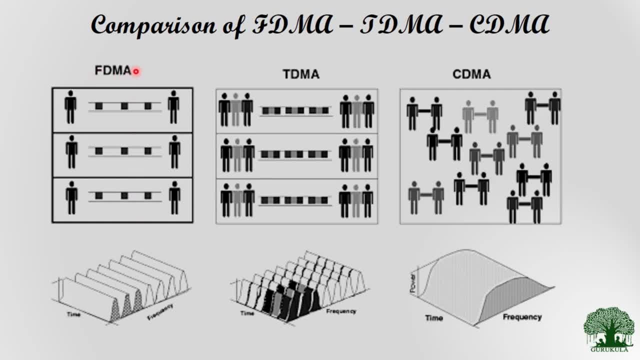 transmission is possible with fdma systems. and secondly, we have seen tdma, that is, time division, multiple access- where there is literally no restrictions on the frequency band, but entire frequency band will be accessed by a particular user, but only for a particular period of time. so 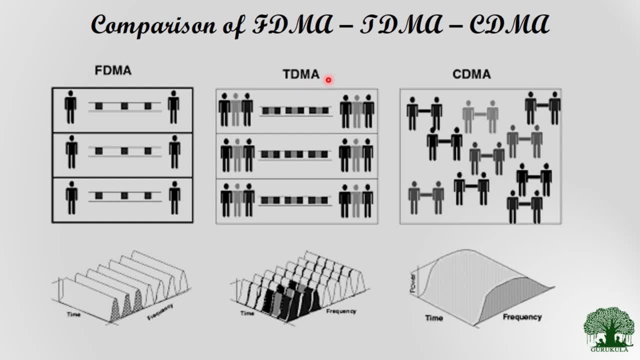 continuous transmission is not possible in case of tdma systems. but the advantage of the fdma system is he can use the entire frequency band so that any um, any level of bandwidth, if even the user has higher bandwidth of signals to transmit, he could able to transmit in the time division multiple. 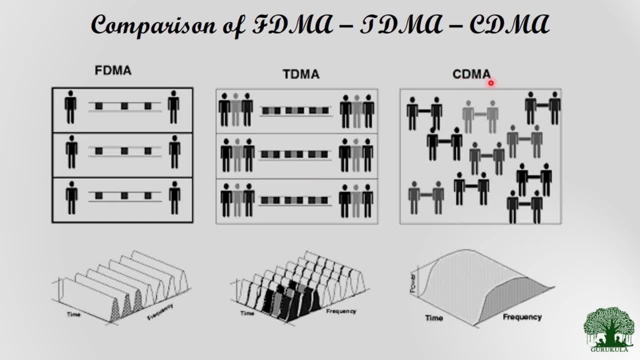 axis system. so when the finally, today we have seen code division, multiple axis, where user doesn't have any restrictions on the frequency and as well as time, so which will help us to achieve higher data rates, but the uses are differentiated with respect to code, so each and every user will be 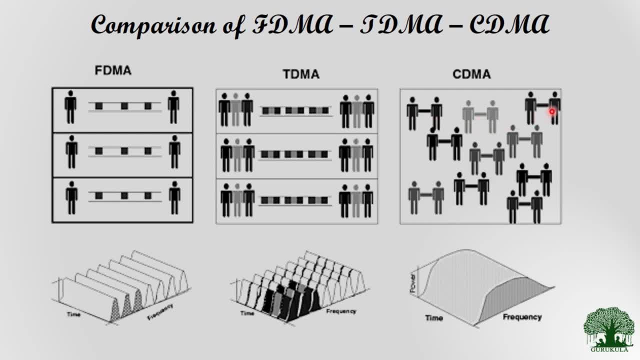 allocated a different code so that the user can use the entire frequency band so that any level of frequency of connections could pick up at the same time. so that was written in개어칵계IANJ SA- we, and it is understood that all the codes have to be maintained at.